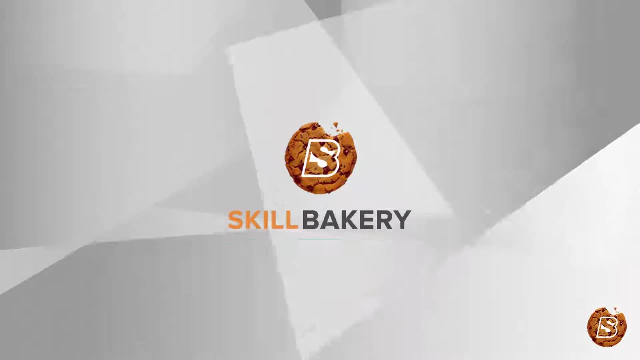 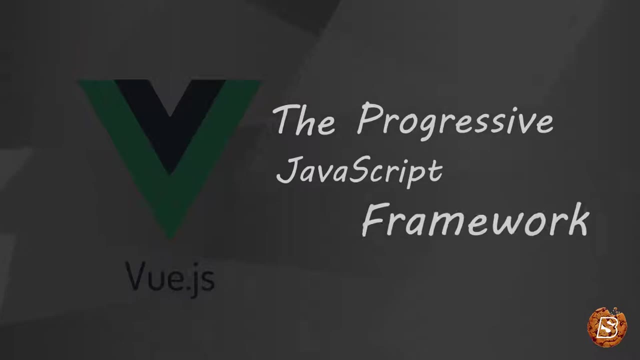 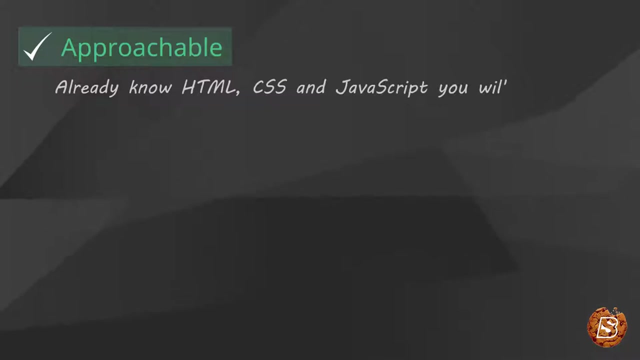 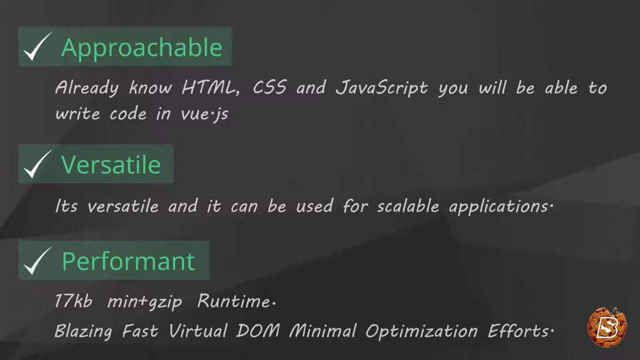 Welcome to learning Vuejs, the progressive JavaScript framework. It's approachable. If you already know HTML, CSS and JavaScript, you will be able to write code in Vuejs. It's versatile and it can be used for scalable applications. The size of this library is just 17 kilobytes when minified and it gives you blazing fast virtual DOM with minimal optimization efforts. So let me formally introduce you to Vuejs framework. 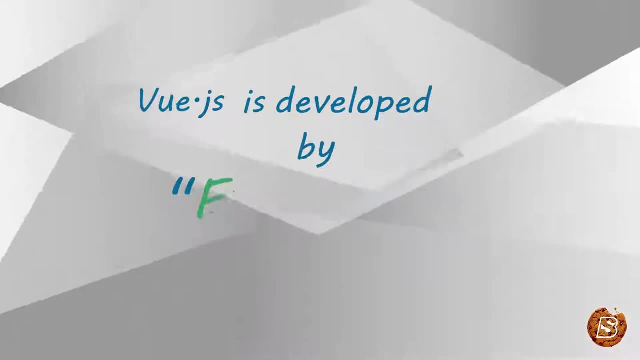 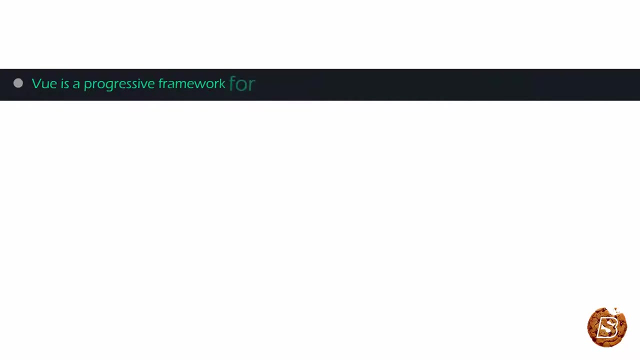 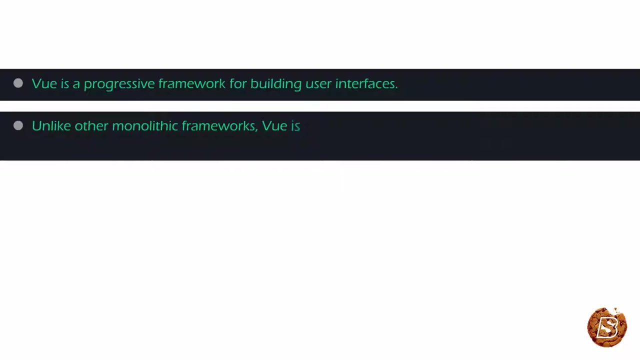 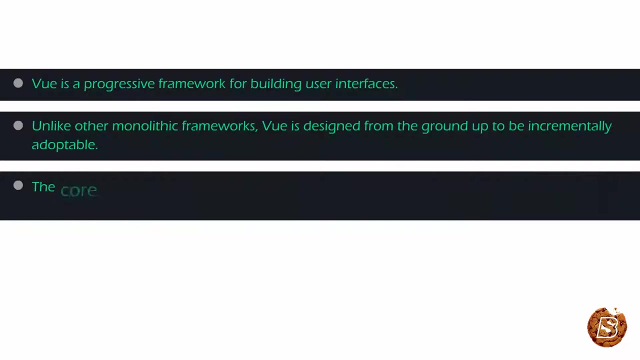 Vuejs is developed by Ivan Yu. Vuejs is a progressive framework for building user interfaces. Vuejs is a progressive framework for building user interfaces. Unlike other monolithic frameworks, Vuejs is designed from the ground up to be incrementally adaptable. The core library is focused on the Vuejs layer only and it's very easy to pick up and integrate with other libraries or existing projects. 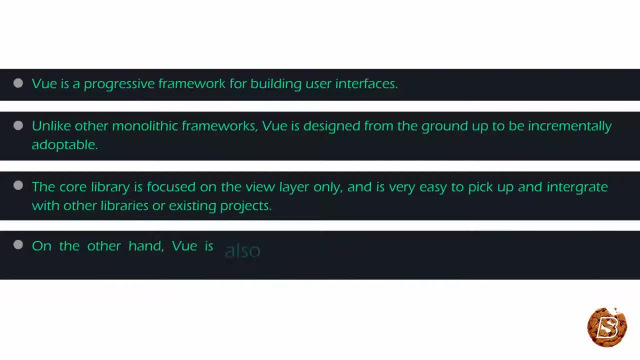 On the other hand, Vuejs is also perfectly capable of powering sophisticated single-page applications when used in combination with modern tooling. On the other hand, Vuejs is also perfectly capable of powering sophisticated single-page applications when used in combination with modern tooling. 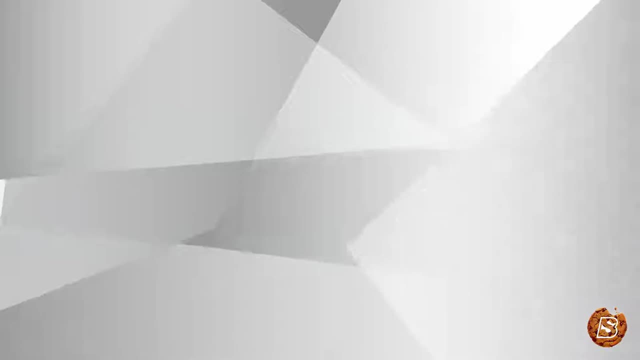 In fact, Vuejs is one of the biggest gatekeepers in Vue development in來 world. The message of this specific course is true to community: comradebracht: If you are totally new to front end development, go and download these materials and see how they are used in it. 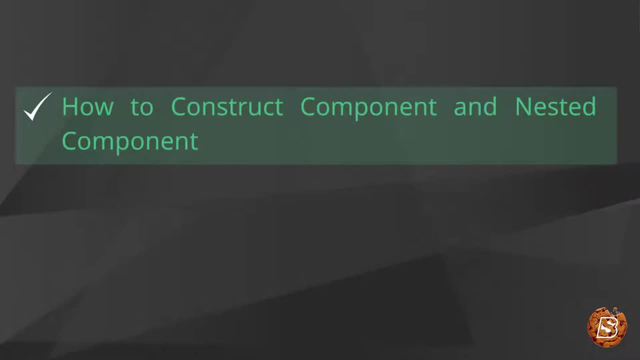 In this course we will be0001 engineer, basically understanding of how to construct components and nested components. See how Vuejs brilliantly keeps the everybody wrộing and evolving through different gab rival gatekeepers to create innovation, to conf economistsance to höher. the distribution of entries for Türk masters and all 2018 papers for on campus and articles. population of groups presented. 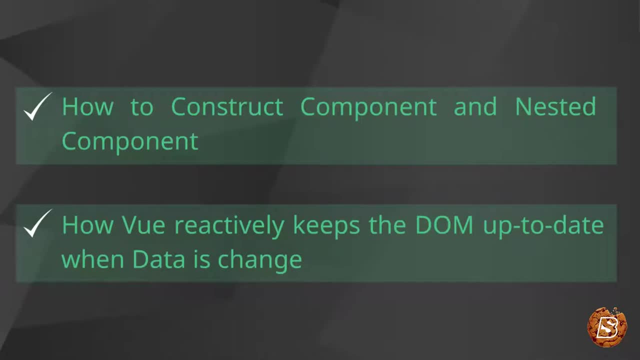 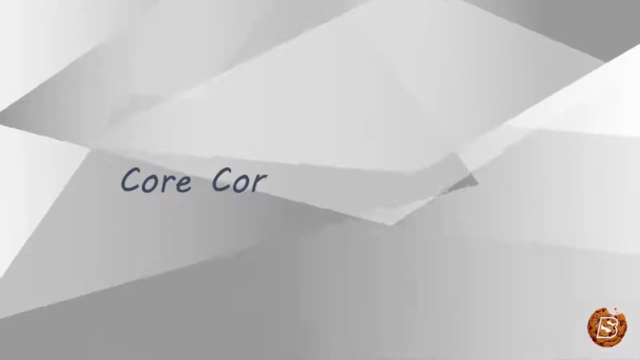 and see how Vuejs reactively keeps the massacre of users out ofiennent. So that's an example of engineering this event. Thank you, DOM. up to date when data is changed. apart from that, we'll be also covering on other core concepts of Vuejs, like template, syntax, computed properties. 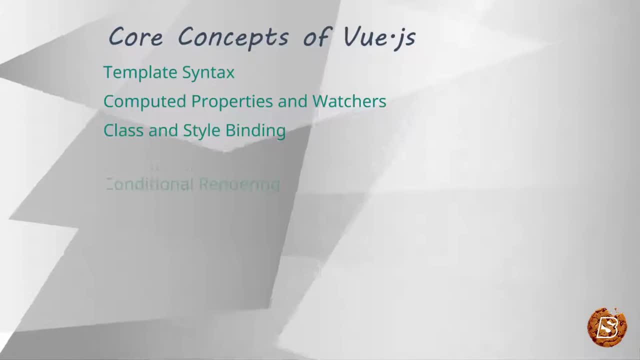 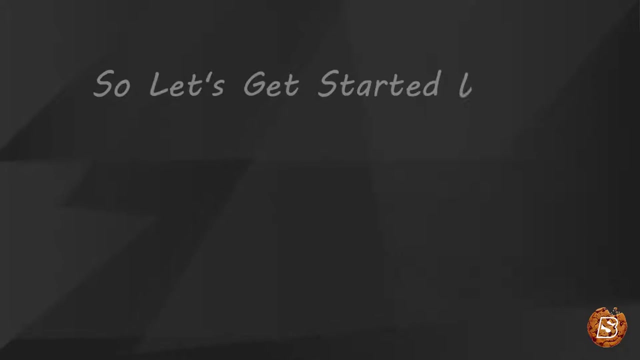 and watchers, class and style bindings, conditional rendering, list rendering, event handling, form, input bindings. We'll also be covering on routing, state management, rendering and custom directives. So let's get started with learning Vue.